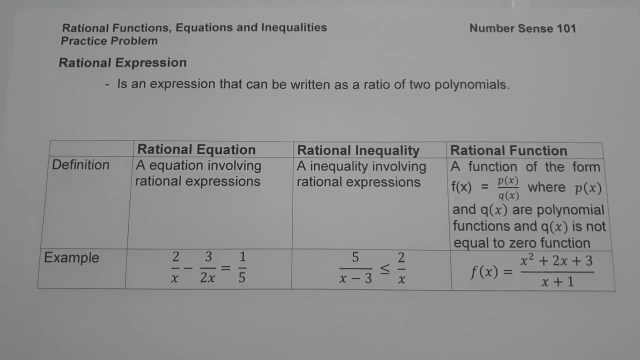 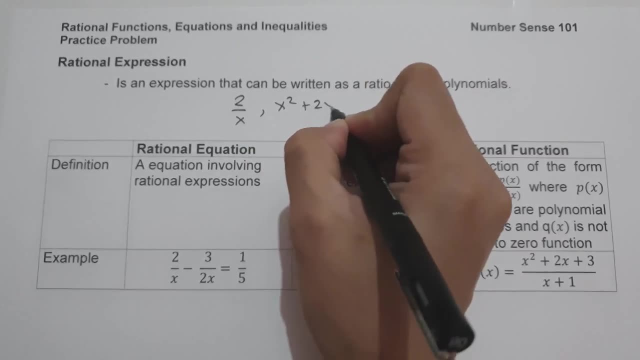 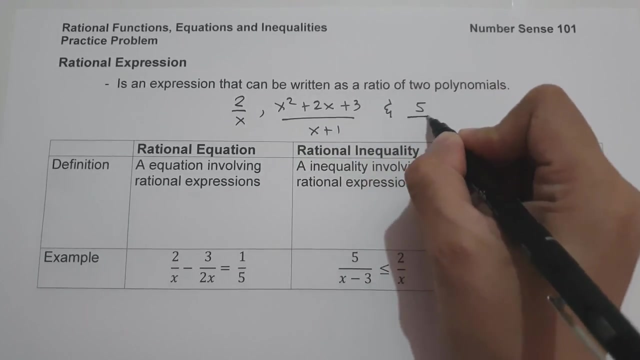 it is an expression that can be written as a ratio of two polynomials. For example, let's say we have 2 over x, x squared plus 2x plus 3, all over x plus 1.. Let's say we have 5 over x minus. 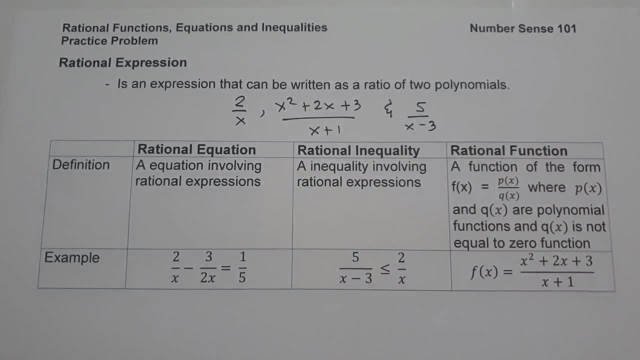 3.. So those are the examples of rational expression, because they are written in the ratio of two polynomials. Now let us define what is a rational equation: rational inequality and rational function. So when we say rational equation, it is an equation involving rational 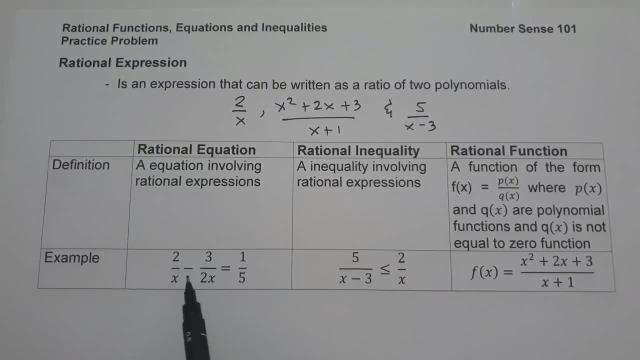 equation. So when we say rational equation, it is an equation involving rational equation. For example, 2 over x minus 3 over 2x equals 1 over 5 is an example of rational equation. And when we say rational inequality, it is an equality involving rational expression. 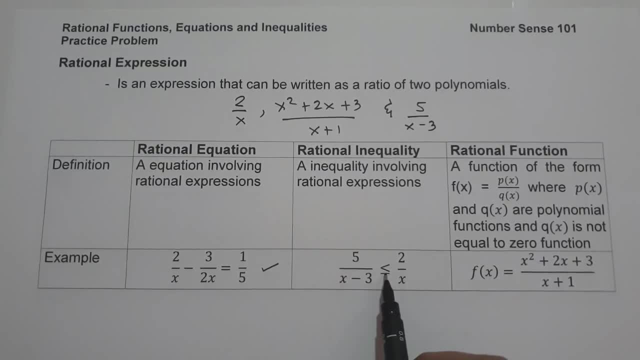 So we have 5 over x minus 3, less than or equal to 2 over x. So this one is an example of rational inequality and the inequality symbol is less than or equal to. So whenever you have an inequality symbol, the given example is rational inequality. And lastly, we have rational function. So when 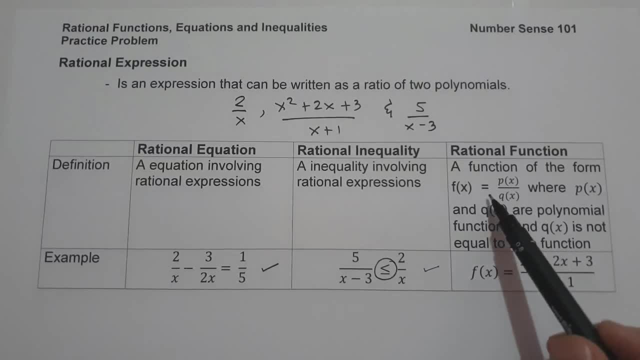 we say rational function. it is a function in the form of f of x equals p of x over q of x, where p of x and q of x are polynomial functions and q of x is not equal to 0. For example, f of x equals x squared plus 2x plus 3, all over x plus 1.. Or it can be written as: y equals x squared. 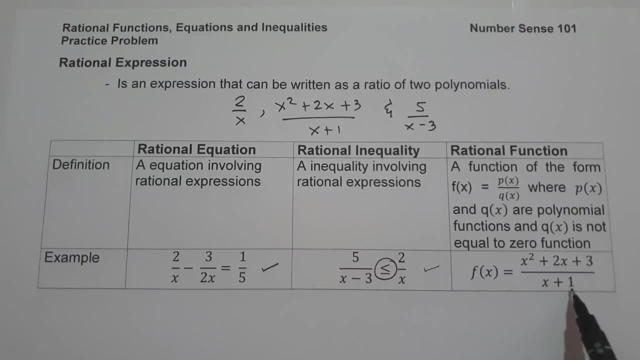 equals x squared plus 2x plus 3, all over x plus one. Or it can be written as: y equals x squared plus 2x plus 3, all over x plus 1.. So those are the basic concepts that we need to understand in. 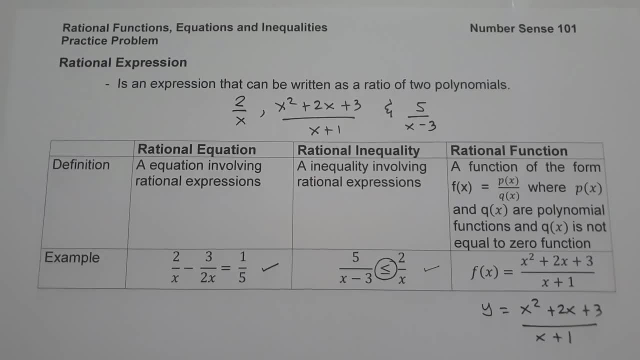 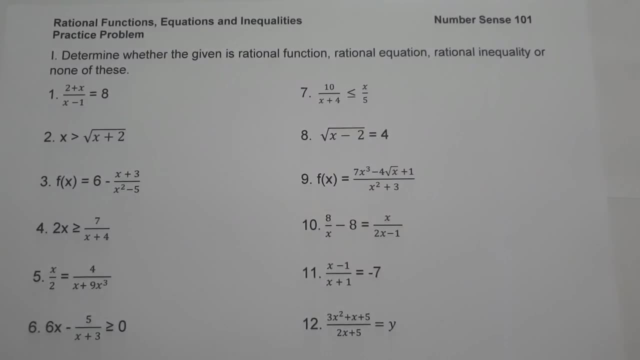 order for us to determine whether the given is a rational functions, rational equations and rational inequalities. So let's start and let's have an example. So let us answer the following set of questions by determining whether the given is a rational function, rational equation, rational inequality or none of this. On number 1, we have 2 plus x, all over. 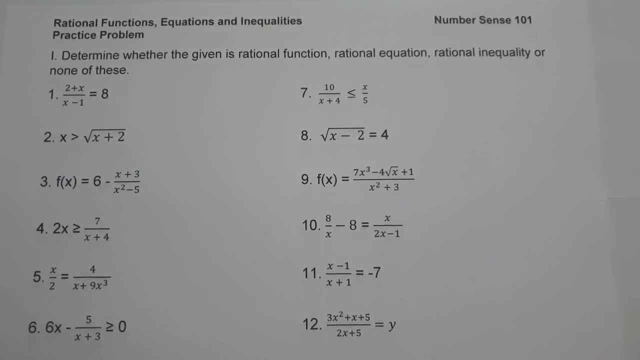 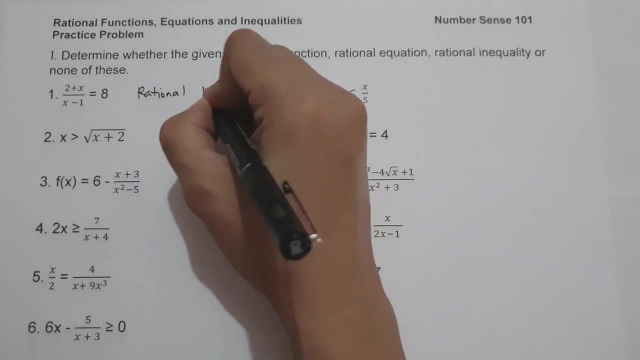 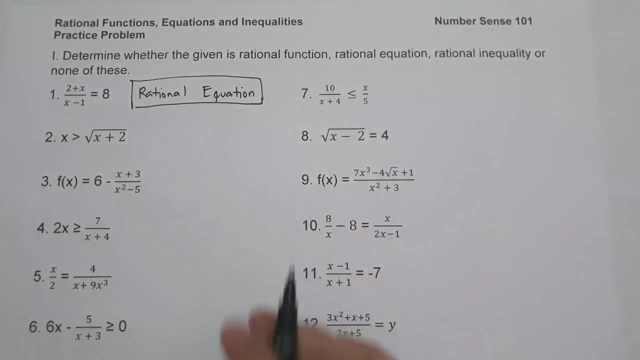 x minus 1 equals 8.. Since we have an equation involving rational expression, our answer will be: rational equation On number 2, x greater than square root of x plus 2.. Since we have a radical sign, and whenever we have a radical sign or expression raised, 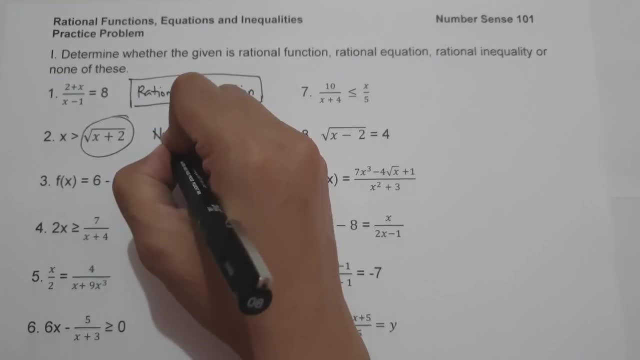 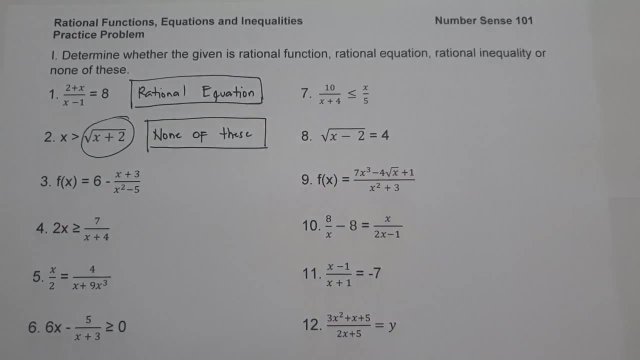 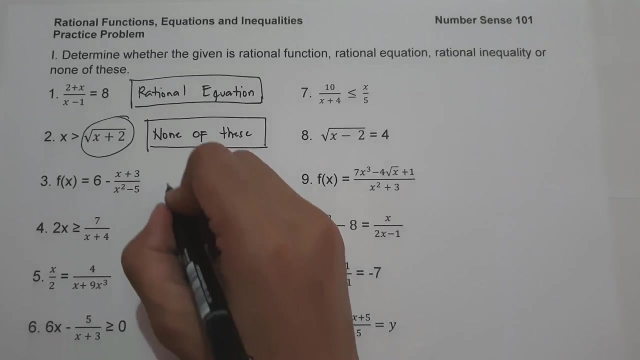 in a fractional exponent, our answer will be none of this. On number 3, f of x equals 6 minus x plus 3 all over x square minus 5.. Since number 3 is written in the form of f of x equals p of x over q of x. our answer on number 3 will be: 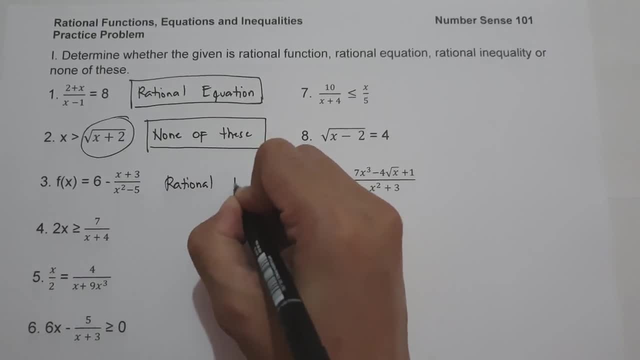 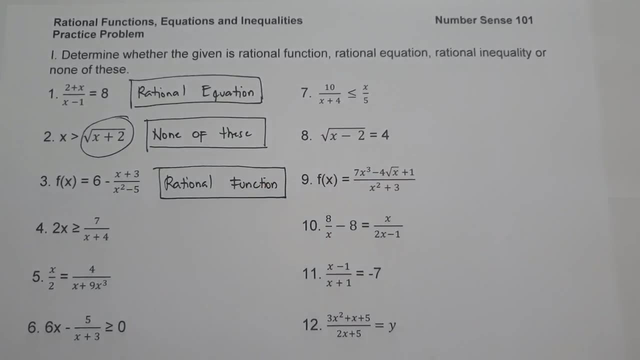 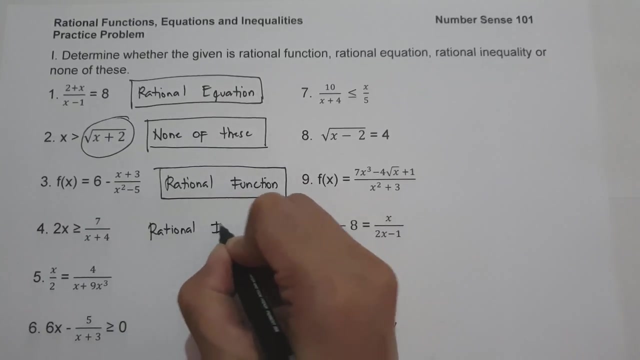 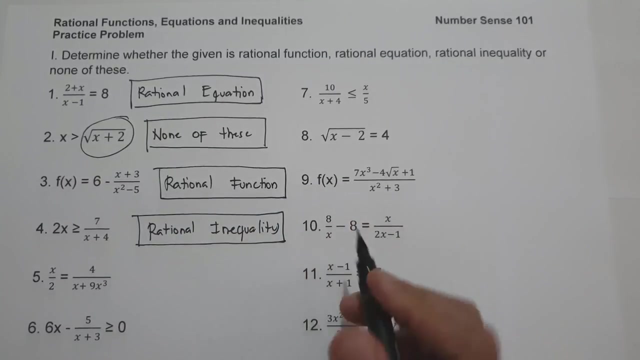 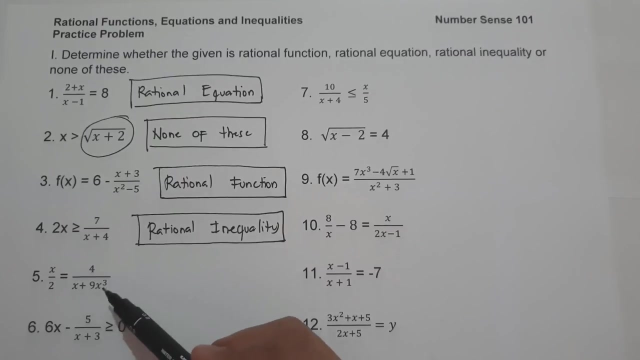 rational function On number 4, 2x greater than or equal to 7 over x plus 4.. Since we have an inequality involving rational expression, our answer will be rational inequality. What about number 5?? We have x over 2 equals 4 over x plus 9x, cubed. Since we have an equation. 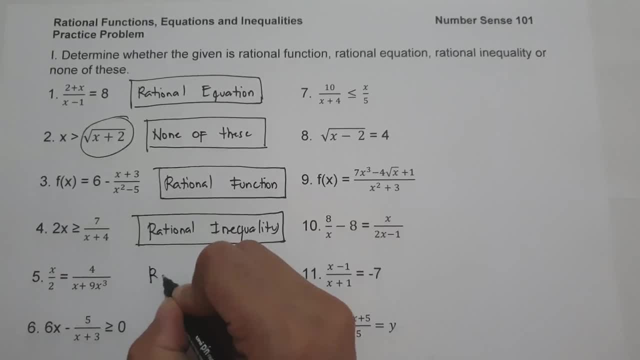 involving rational expression. our answer will be rational equation On number 6, 6x minus 5 over x plus 3, greater than or equal to 7 over x plus 9x, cubed, Since we have an inequality symbol, at the same time we have an inequality involving 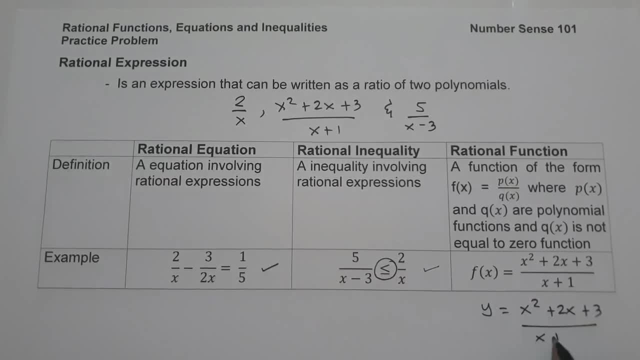 plus 2x plus 3, all over x plus 1.. So when we say rational function, it is an equation involving rational inequality, and the inequality symbol is less than or equal to 2x plus 3, all over x plus 1.. 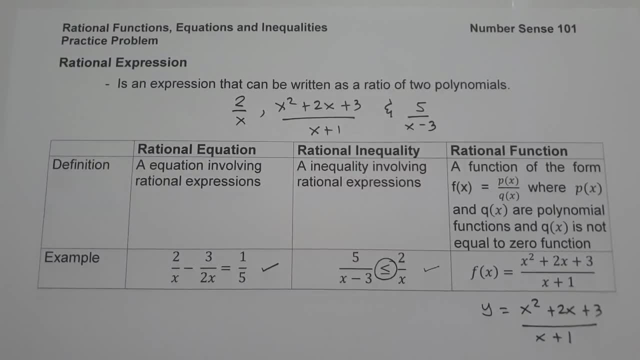 So those are the basic concepts that we need to understand in order for us to determine whether the given is a rational functions, rational equations and rational inequalities. So let's start and let's have an example. So let us answer the following set of questions by determining: 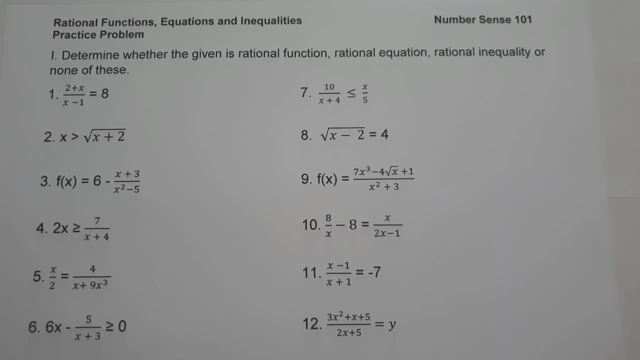 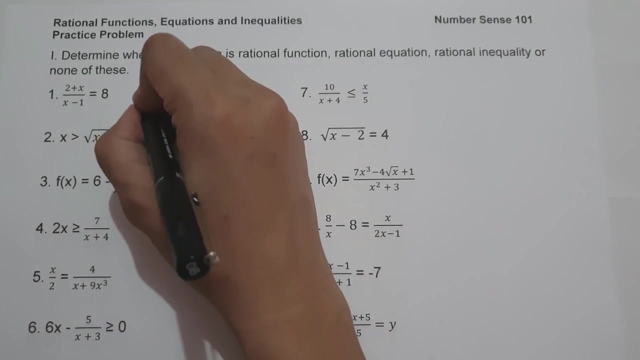 whether the given is a rational function, rational equation, rational inequality or none of this. On number one, we have 2 plus x, all over. x minus 1 equals 8.. Since we have an equation involving rational expression, our answer will be rational equation. 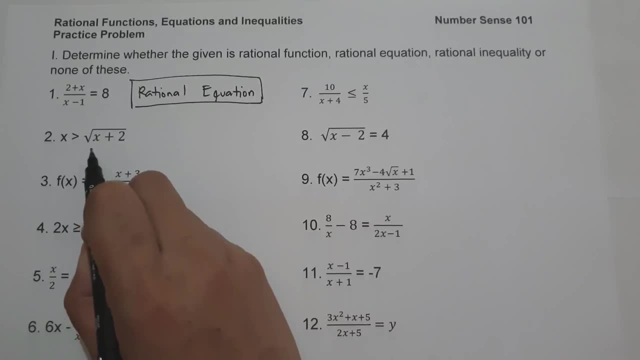 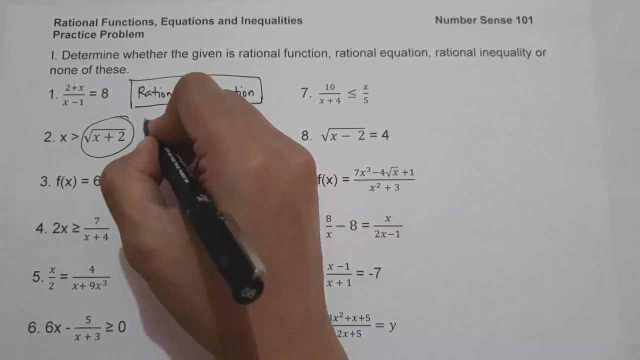 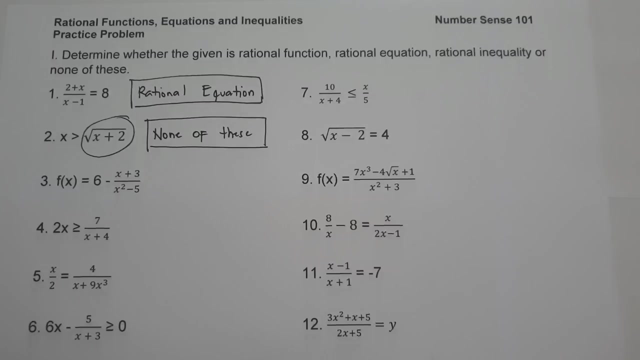 On number two: x greater than square root of x plus 2.. Since we have a radical sign, and whenever we have a radical sign or expression raised in a fractional exponent, our answer will be none of this. On number three: f of x equals 6 minus x plus 3, all over x square minus 5.. Since number three 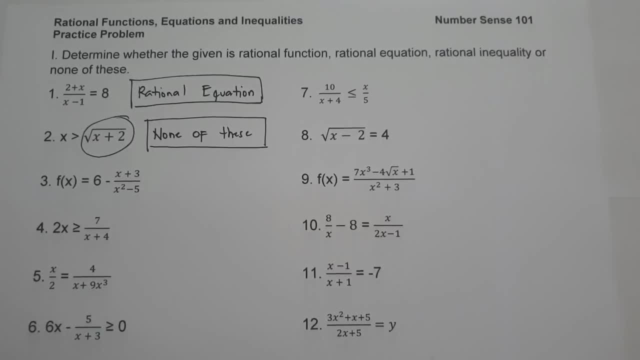 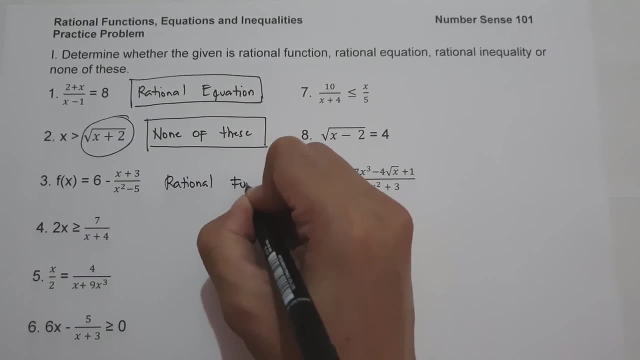 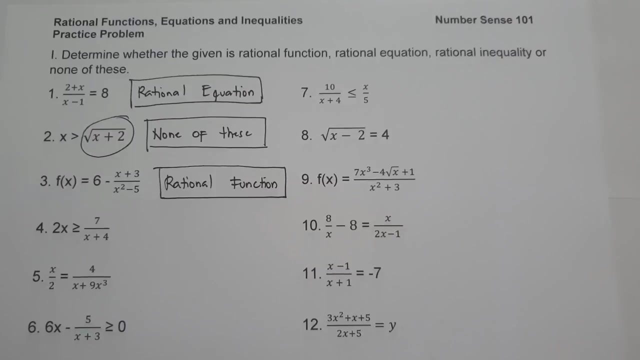 is written in the form of f of x equals p of x over q of x. our answer on number three will be rational function. On number four: 2x greater than or equal to 7 over x plus 4.. Since we have an inequality, 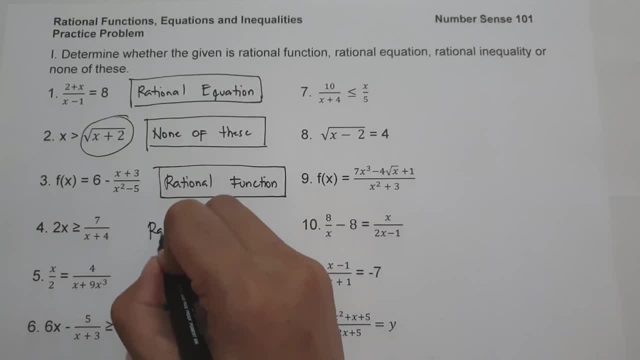 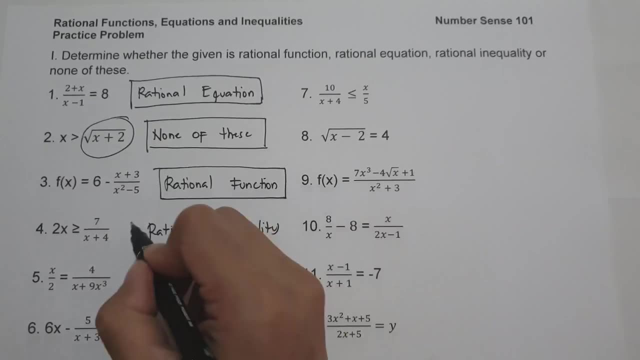 involving rational expression, our answer will be rational inequality. What about number five? We have: x over 2 equals 4 over square root of x plus 4.. Since number three is written in the form of 7 over x plus 4, all over x plus 4.. Since number three is: 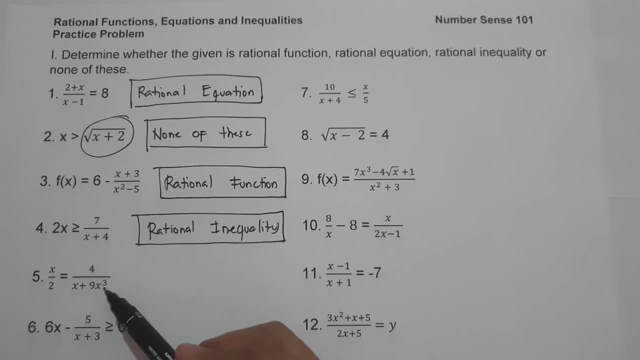 equal to 7 over x plus 4.. Since number three is equal to 7 over x plus 4.. Since number three equals four over x plus nine x cubed. Since we have an equation involving rational expression, our answer will be rational equation. 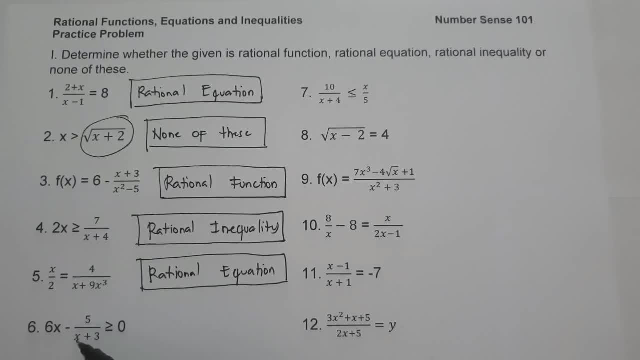 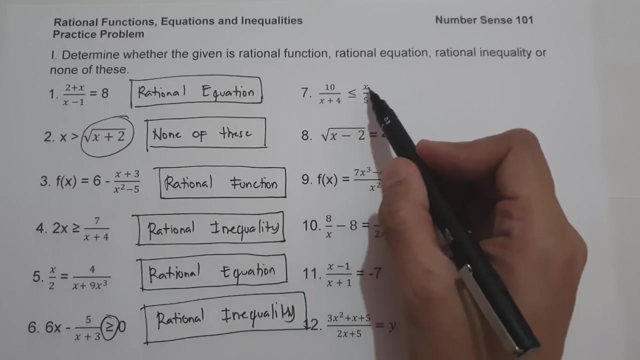 On number six, six x minus five over x plus three greater than or equal to zero. Since we have an inequality symbol, at the same time we have an inequality involving rational expression, our answer will be rational inequality. On number seven, we have 10 over x plus 4 less than or equal to x. 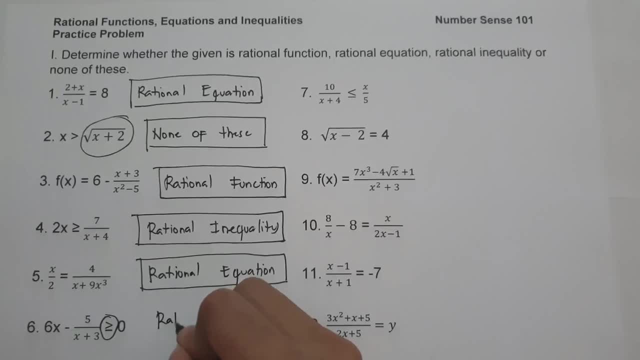 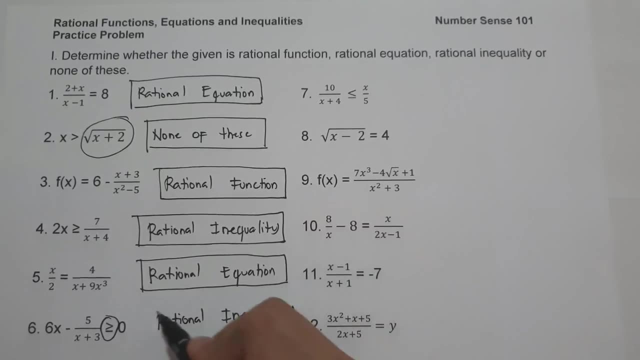 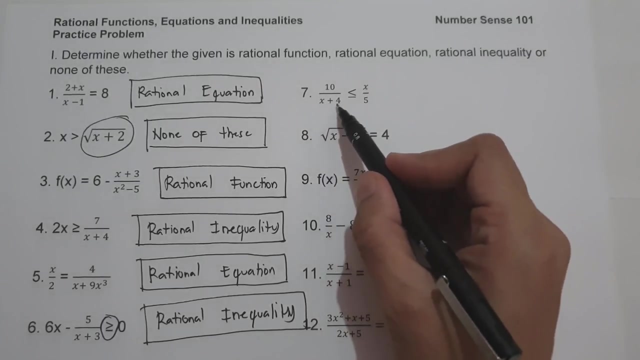 rational expression, our answer will be rational inequality. On number 7, we have 10 over x plus 4, less than or equal to x over 5.. So the inequality symbol is less than or equal to 7 over x plus 4.. Since we have an inequality symbol at the 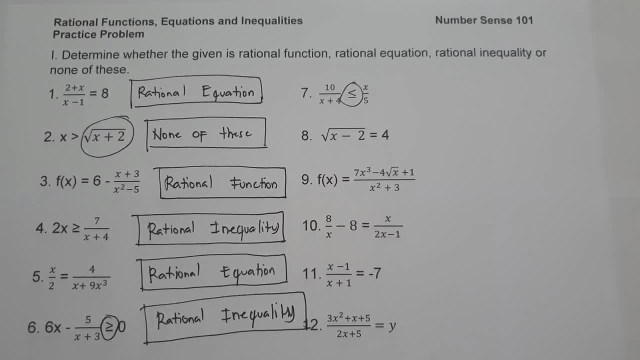 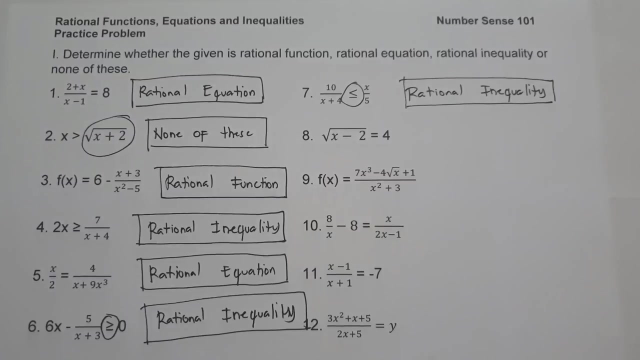 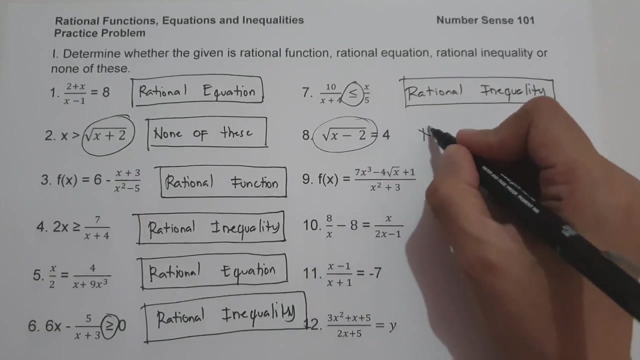 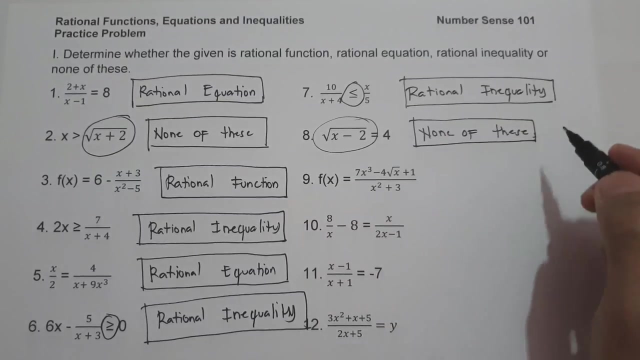 same time, we have an inequality involving rational expression, our answer will be rational inequality. On number 8, we have: square root of x minus 2 equals 4.. Since we have a radical sign, our answer will be none of this. On number 9, f of x equals 7x, cubed minus 4. square root of x plus 1 all over x squared. 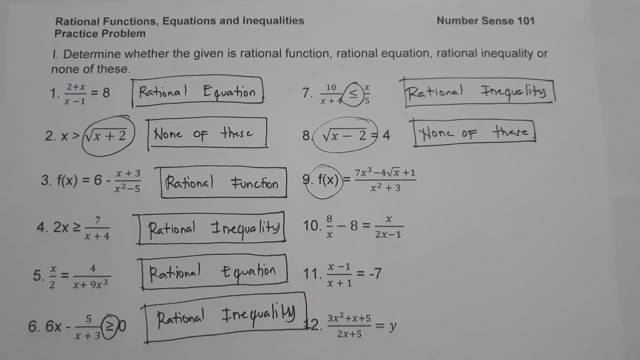 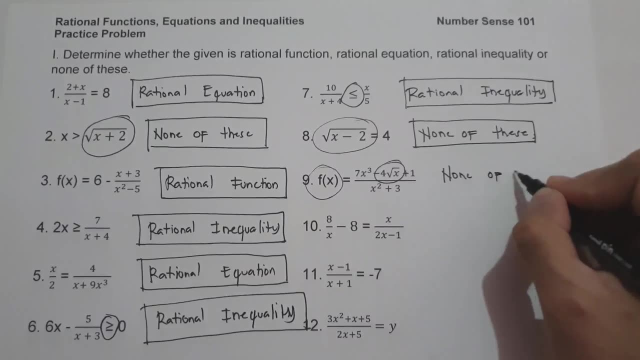 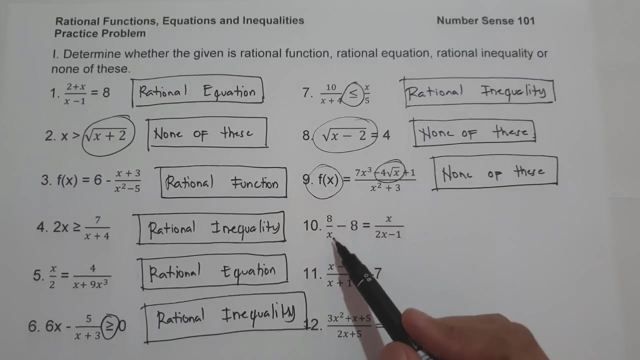 plus 3.. Although we have an f of x, but we still have a radical sign on the numerator, our answer will be none of this. On number 10, we have 8 over x minus 8 equals x over 2x minus 3.. Since we have an inequality, 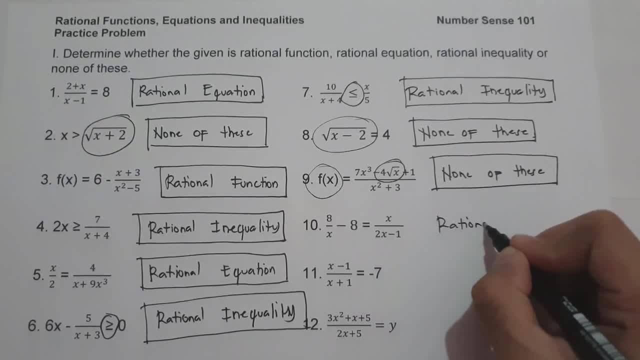 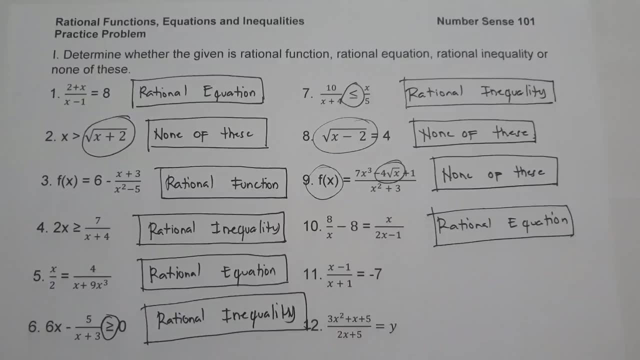 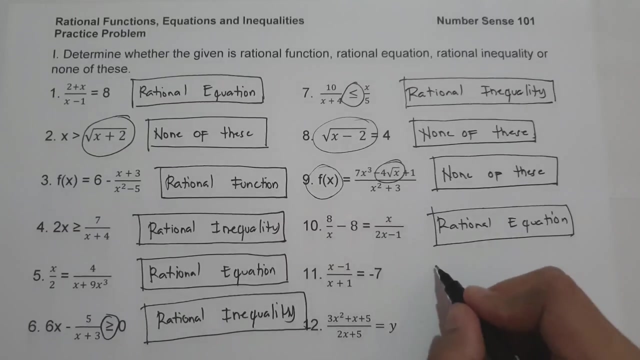 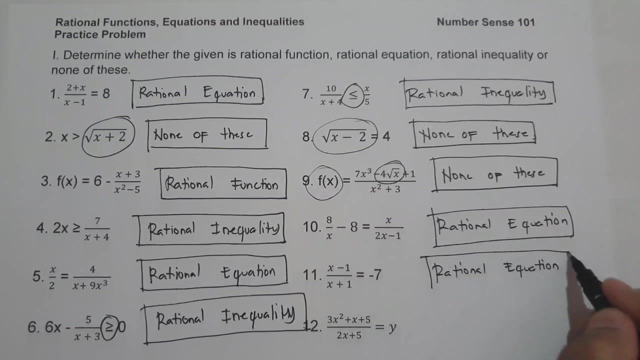 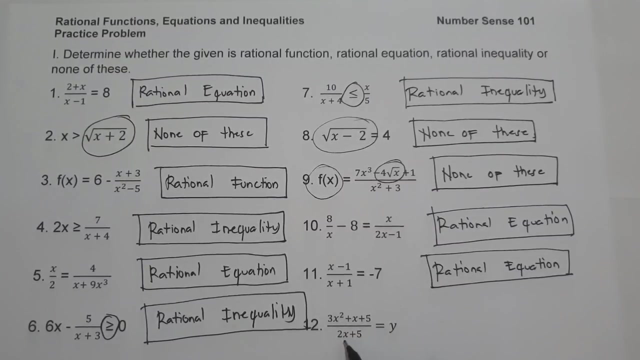 symbol. at the same time, we have an inequality involving rational expression. our answer will be: on number 12, we have 3x squared plus x plus 5 all over. 2x plus 5 equals y. if you are going to write this one, we can have y equals 3x squared plus x plus 5 over 2x plus 5. 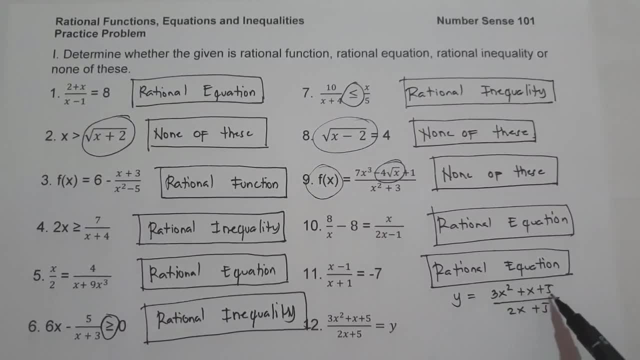 or f of x equals 3x squared plus x plus 5, all over 2x plus 5. since number 12 is written in the form of f of x equals p of x over q of x, our answer on number 12 will be rational function. 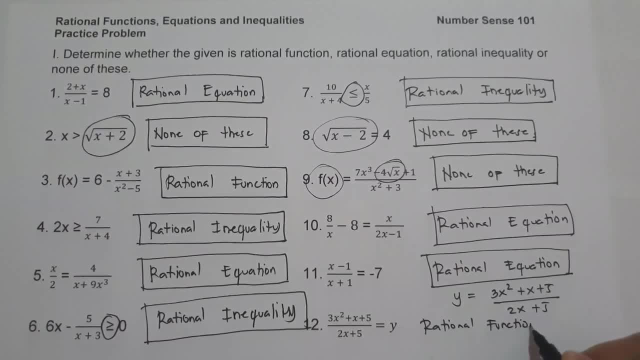 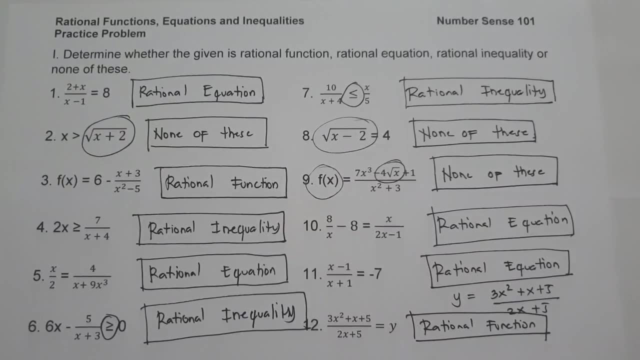 and this will be our answer, so i hope you've learned from this video. thank you so much for watching, and god bless us all. 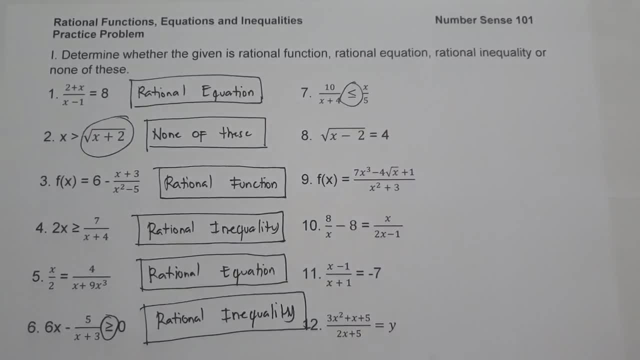 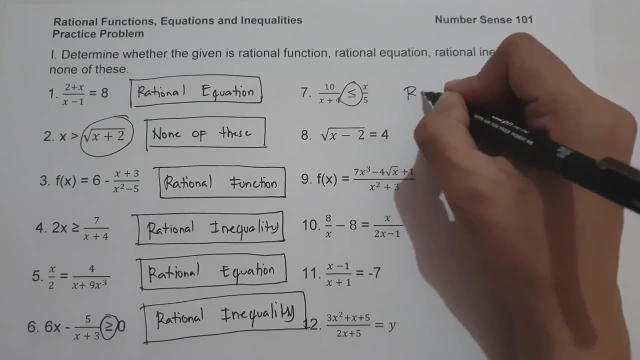 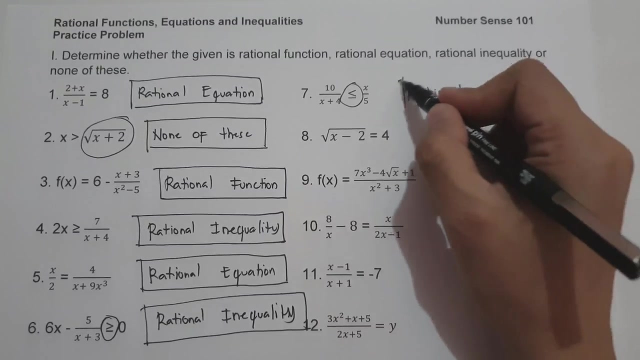 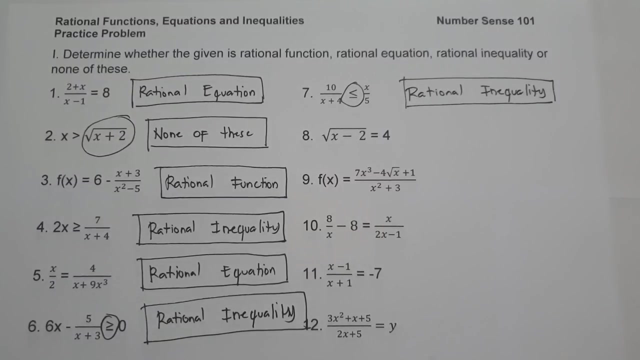 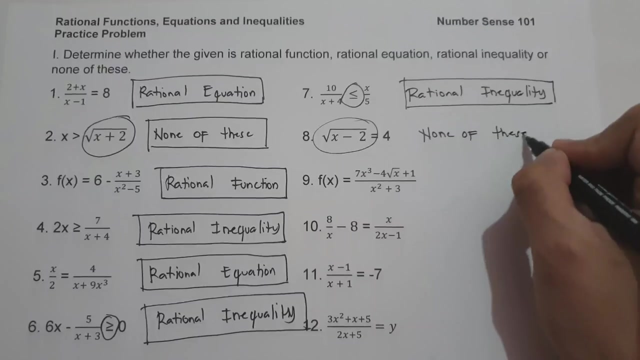 over 5.. So the inequality symbol is less than or equal to and the same time, we have an inequality involving rational expression. our answer On number seven will be rational inequality. On number eight, we have square root of x minus two equals 4.. Since we have a radical sign, our answer will be none of this.